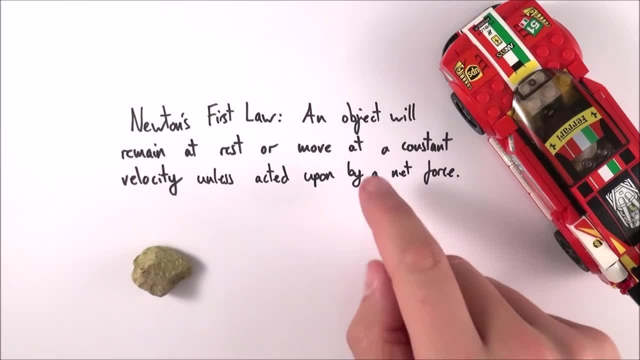 sort of 1687.. So a long time ago. And he basically said that an object will remain at rest or it will move at a constant velocity unless acted upon by a net force. And therefore this space rock that we might consider, if there's no net force acting on it, it will just keep moving. 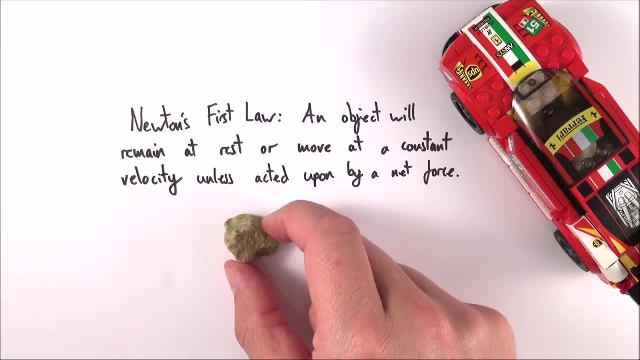 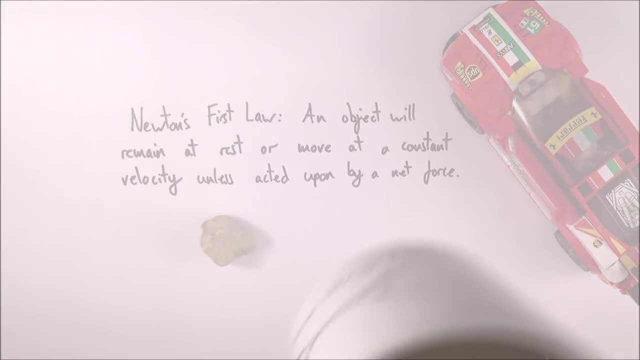 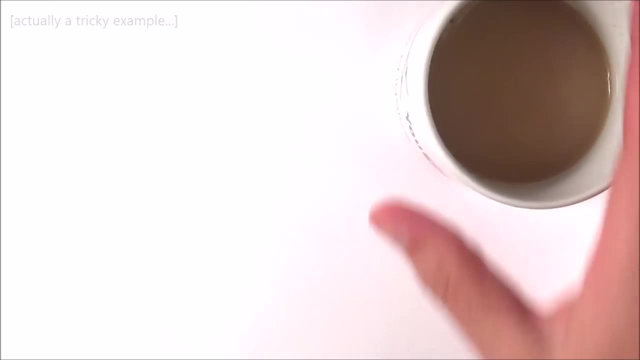 at the same velocity until another force acts on it which might speed it up or slow it down. But what about an example with a cup of tea? Okay, let's think about a nice, straightforward example. Here we have a mug, A mug of tea which is just resting on the table I have down here. 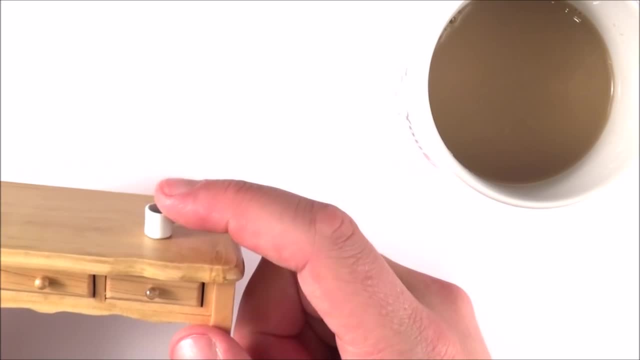 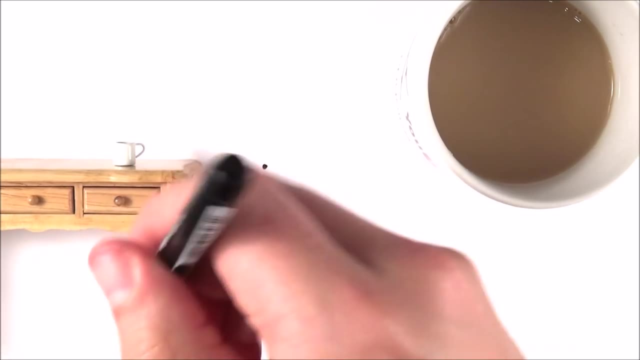 And if we think about what's happening- basically I've got the table and I've got the mug resting on top of it And we can maybe think about the forces which are acting on it- So on this mug there's going to be a downwards force due to gravity, which we call the weight. 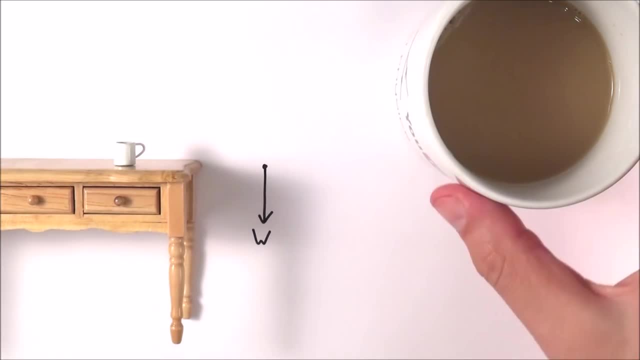 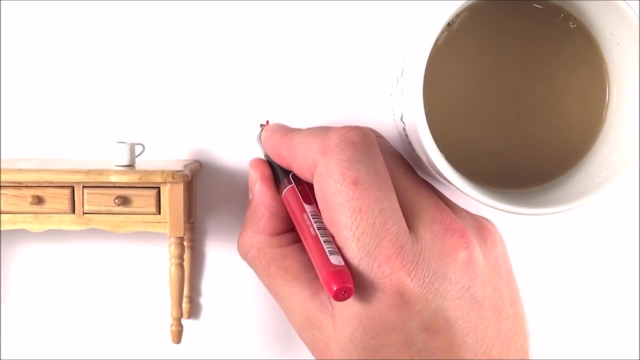 I'm going to call that W for the weight, And the reason that this mug here doesn't fall through the table is because the table is pushing back upwards on it, And this is what we call a reaction force, Sometimes called the normal, sometimes called the contact. 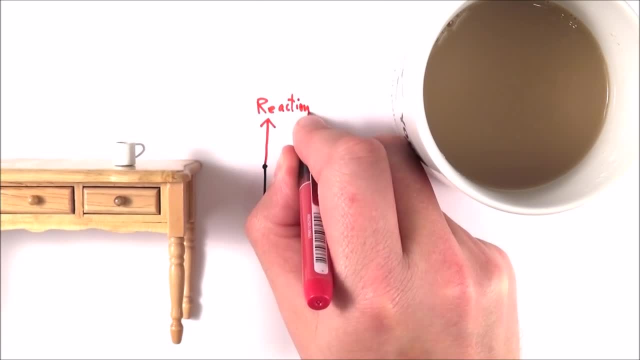 I'll just call it the reaction over here And put simply: at GCSE we say that the reaction force is equal to the weight, But in actual fact that's not necessarily true. The reaction force, it isn't equal to the weight force. 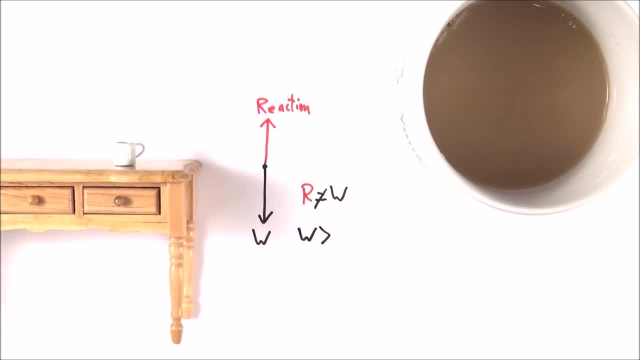 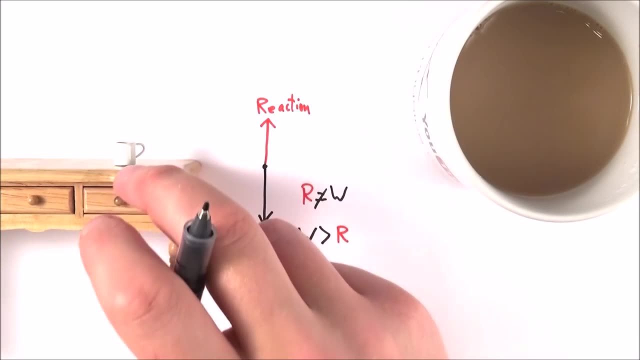 In actual fact, the weight is going to be bigger than the reaction. Why is that? Well, it's because this object here is not stationary, Although it might look still here, And especially compared to, maybe in reference to, the camera that we have up there. 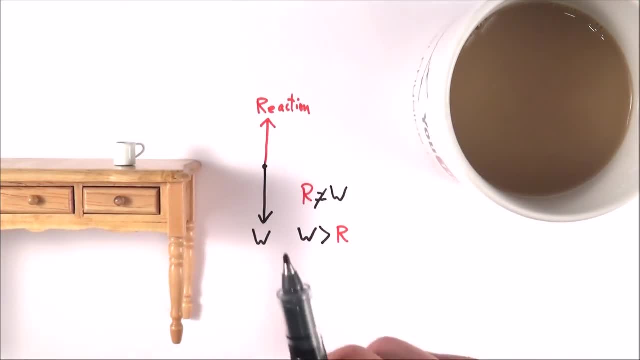 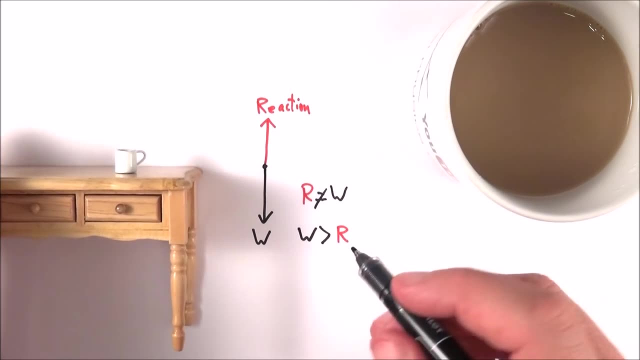 up here. if we sort of- maybe sort of- zoom out and zoom out, we find that actually this table and the mug are on the earth and the earth is spinning round. That means there needs to be a centripetal force which is acting inwards, that stops this moving off into space. 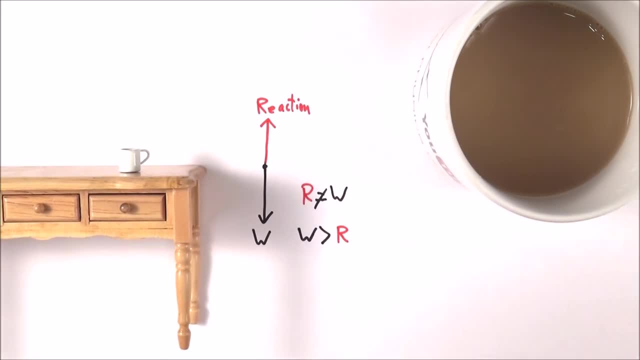 So because the weight is bigger than the reaction. that means, when we look at these two forces, there's effectively a net force which is acting downwards, and it's this net force here which provides a centripetal force. Now, does that go against Newton's first law you know about?